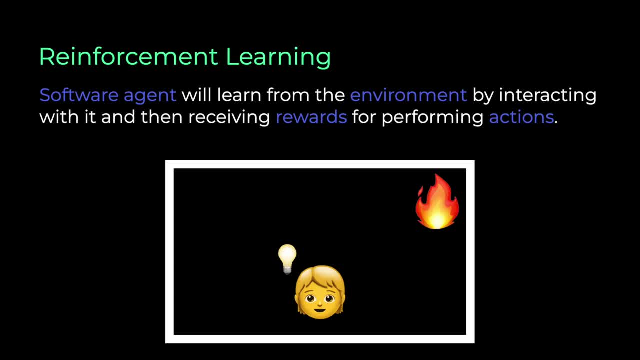 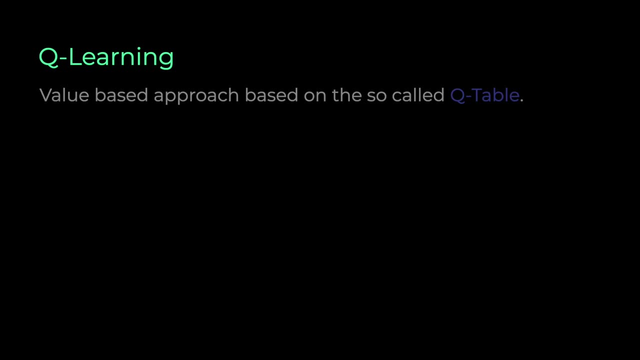 careful and not get too close. And this is exactly how reinforcement learning works. It's the computational approach of learning from actions in an environment through rewards and punishments. One specific implementation of this approach is the Q-learning algorithm. It's a value-based approach based on a so-called Q-table. The Q-table calculates the maximum. 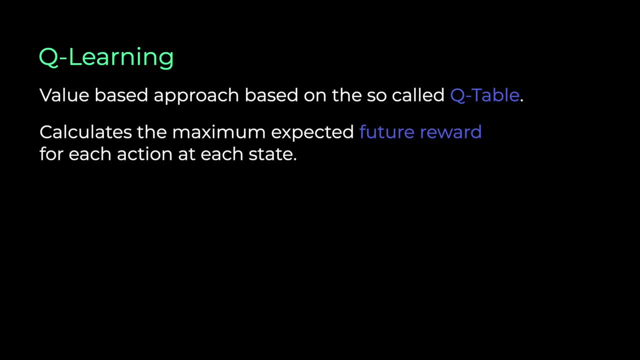 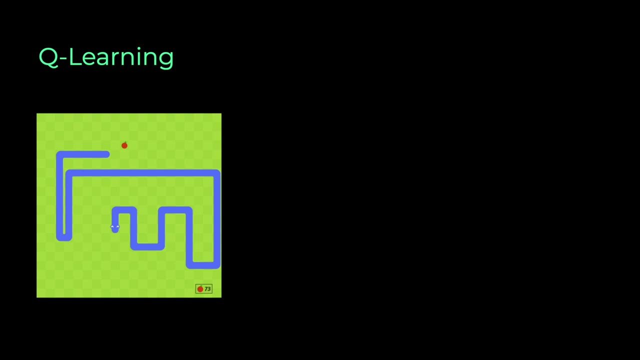 expected future reward for each action at each state, And with this information we can then choose the action with the highest reward. Let's look at a concrete example to make this more clear. Let's say we want to teach an AI how to play the snake game. In this game, the snake tries to reach and eat the food. 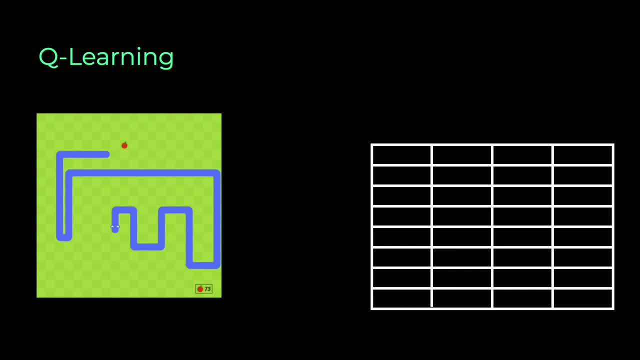 without hitting the wall or itself. We can list the actions and states in a Q-table. The columns will be the four possible actions. the snake can do turning left right up and down, And the state can be the current direction, so also left right, up and down. 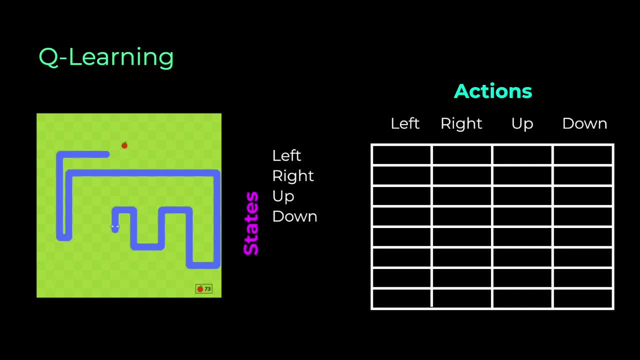 These are the rows, But of course we can add more states to describe the current situation. For example, we can describe the location of the food and add the states food is left of the snake right up or down. We could also do the same thing with the walls and describe the danger, but for simplicity, 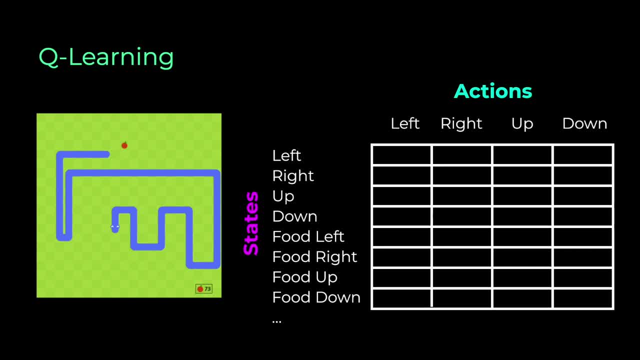 I leave this out here. But you see, the more states we add here, the more information we have about the environment, but also the more complex our system will get. Okay, so now we have all rows and columns and now the value of each cell will be the. 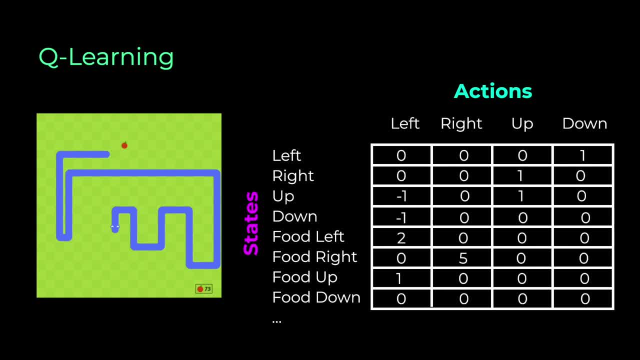 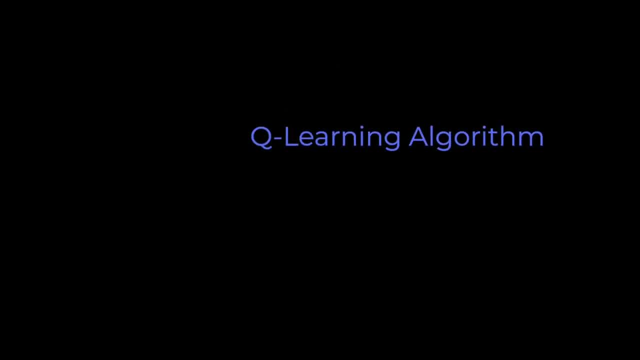 maximum expected future reward for that given state and action. We call this the Q-value. So far, so good. But how do we calculate this Q-value? Here's the interesting part: We do not implement this Q-value calculation in a fixed way. Instead, 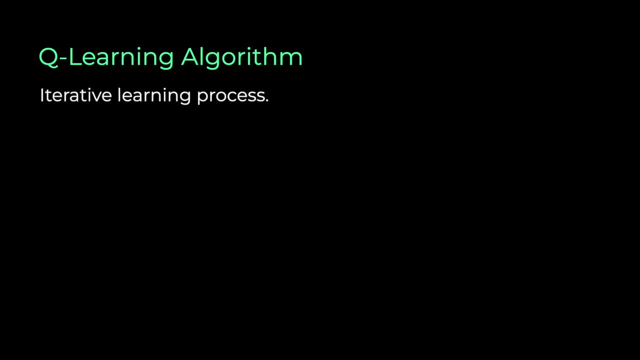 we improve this Q-table in an iterative approach. This is basically our training or learning process. The Q-learning algorithm works like this: First we initialize all Q-values, for example with a zero, Then we choose an action. in the current state This is based. 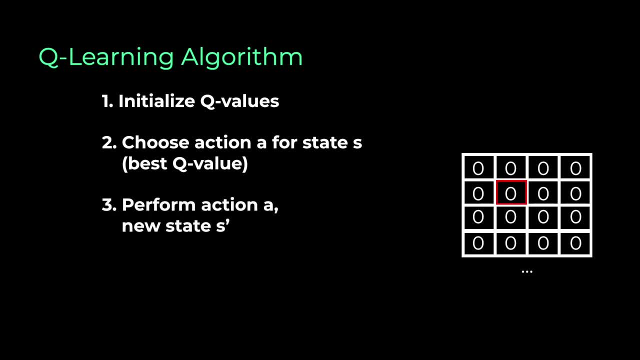 current best Q value. We perform this action and observe the outcome so we get a new state. We also measure the reward after this action And then we update Q with an update formula that is called the Bellman equation. And then we repeat steps 2 to 5 until the learning. 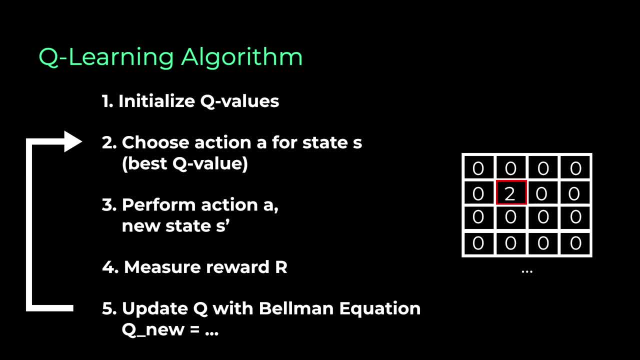 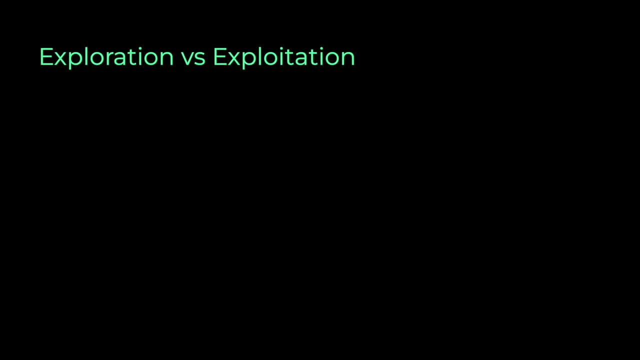 no longer improves and we get a nice Q table in the end. Now a few questions may appear. First, how can we choose the best action in the beginning when all our values are zero? This is where the exploration vs exploitation trade-off comes into play. In the beginning, we choose the action randomly so that our agent can. 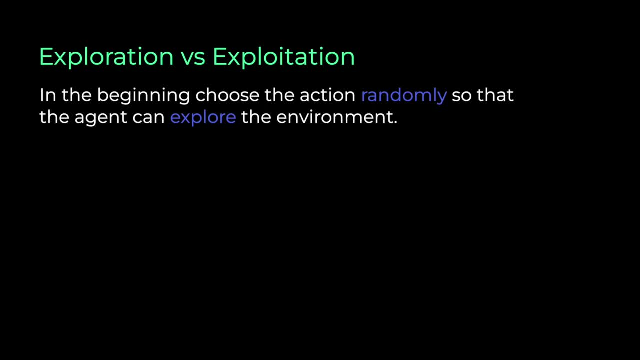 explore the environment, But the more training steps we get, the more we reduce this random exploration and use exploitation instead. So we make use of the information we have. This trade-off is controlled in the calculations by a parameter that is usually called the epsilon parameter. 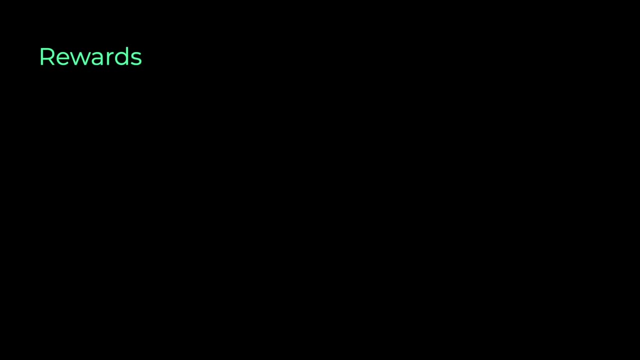 Now the next question. The next question is how the rewards are measured. This is actually up to us, So we can come up with a good reward system for the game. In case of the snake game, for example, we can give a reward of 10 points if the snake eats an apple, and a reward of minus 10 points if 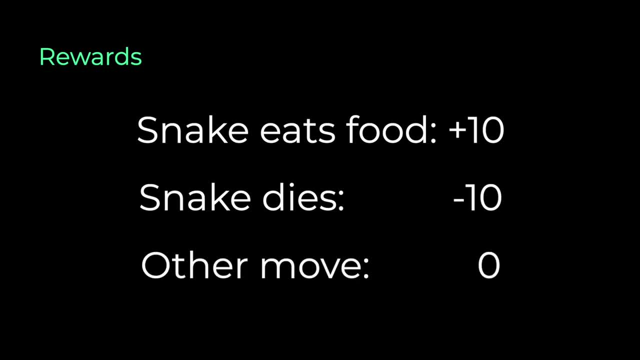 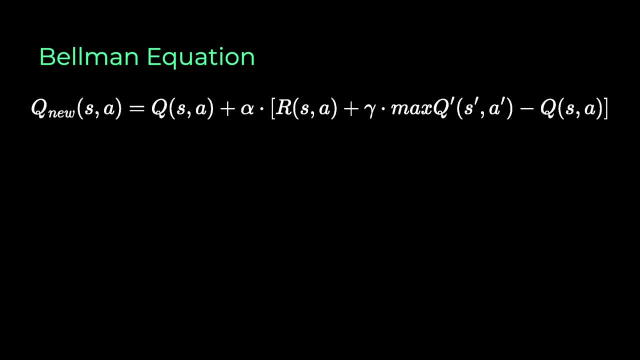 the snake dies and zero for every other normal move. Now, with all these elements, we can inspect the Bellman equation. The idea here is to update our Q value like this: The new Q value is calculated by the current Q value. The new Q value plus a learning rate times a reward, plus a discount rate times the highest. 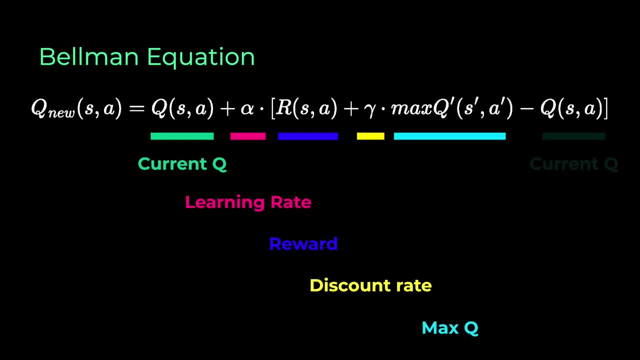 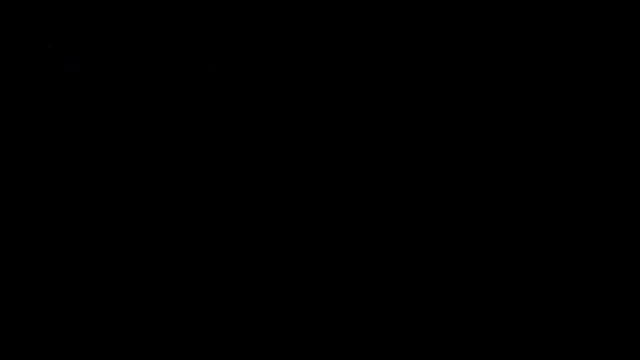 Q value between possible actions from the new state and then minus the current Q value. The discount rate is a value between 0 and 1 and determines how much the agent cares about rewards in the distant future relative to those in the immediate future. So now we have everything we need and, coming back to our iterative learning approach, we 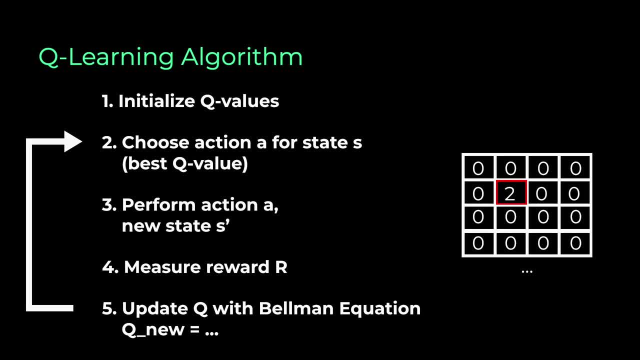 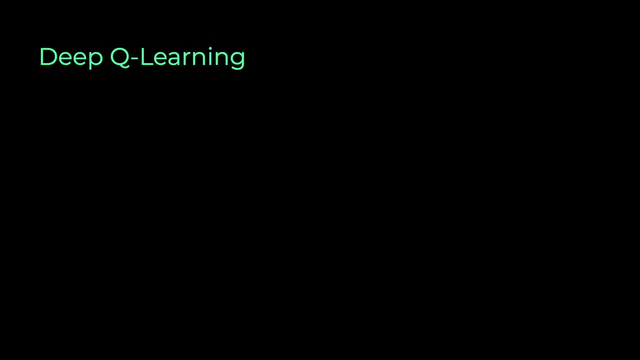 can now come up with a good Q table. Let's start our Q table by using this Q learning algorithm. Now, deep Q learning takes the Q learning idea and takes it one step further. Instead of using a Q table, we use a neural network that takes a state and approximates.